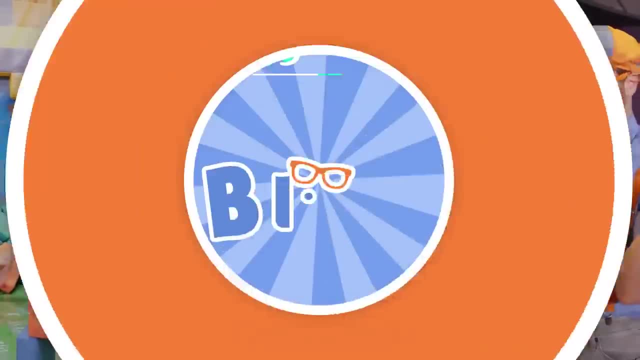 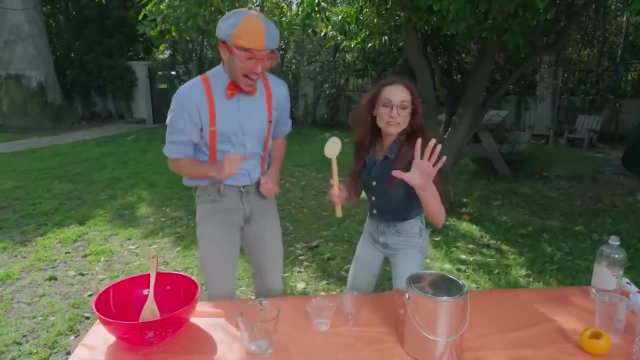 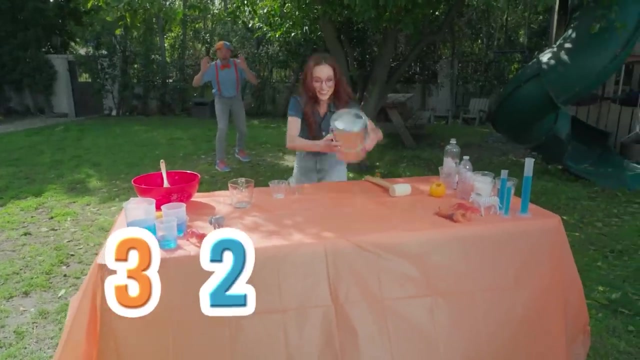 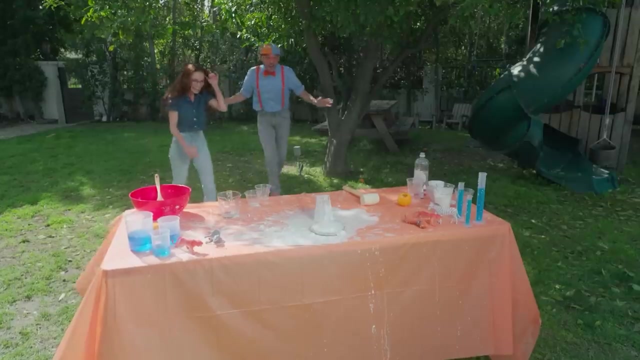 So much to learn about. It'll make you want to shout: Blippi, Everybody, take 10 steps back. We're going to launch in 3, 2, 1!. Whoa, Whoa, Whoa. That was awesome. 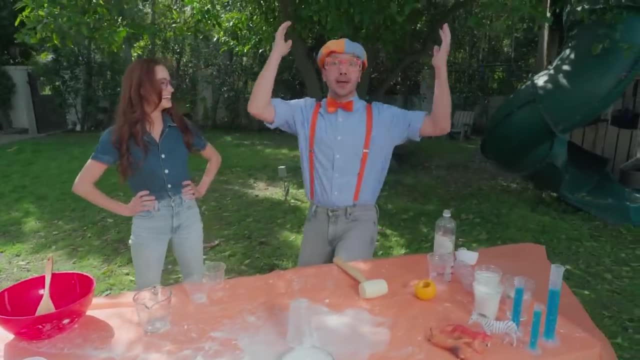 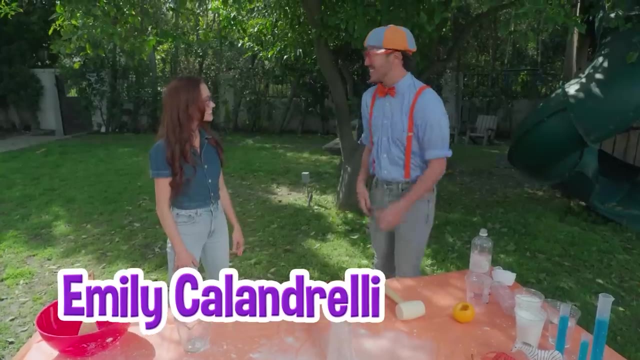 Did you see that paint can shoot up like a rocket? Yeah, Whoa, Hi, I'm Blippi. What's your name? I'm Emily Calandrelli. Nice to meet you. Oh, it's so nice to meet you, Emily. That was an amazing experiment, you did. 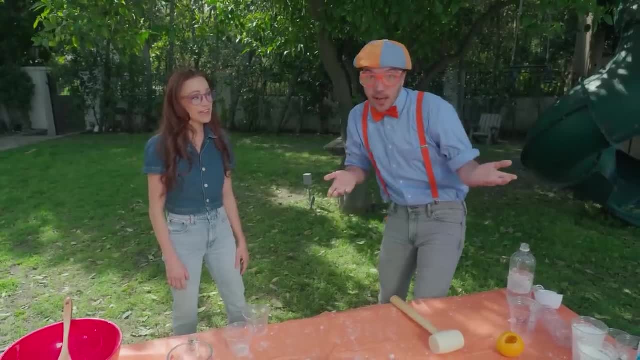 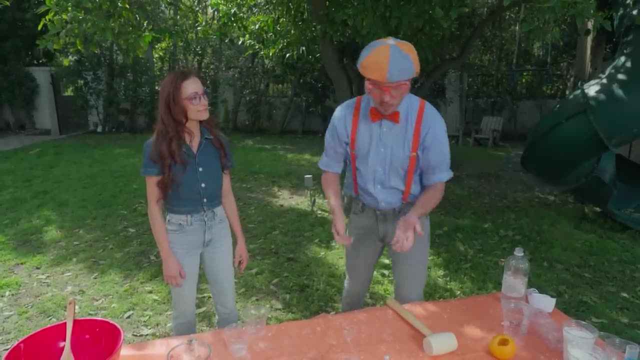 Right. Do you think you could teach us how to do it? I would love to Awesome. Well, wait a minute, Emily. how do you know how to do a science experiment like that? I'm an aerospace engineer, Whoa An aerospace engineer. 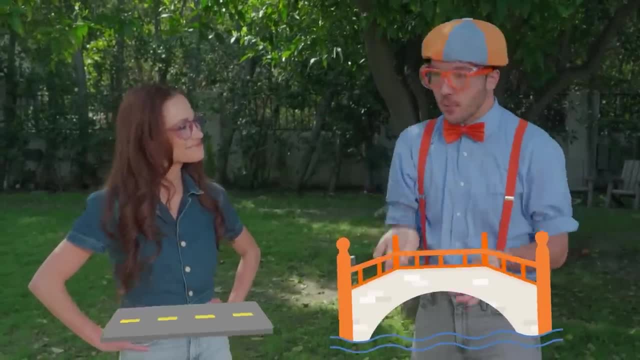 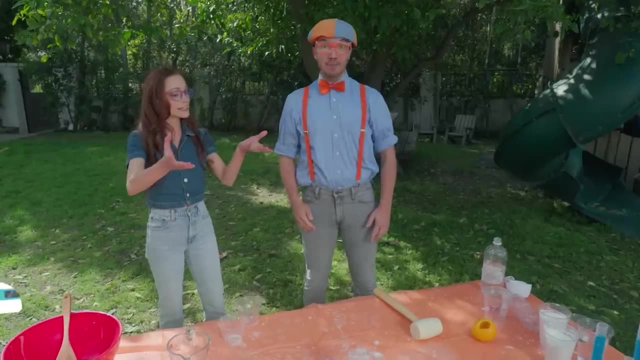 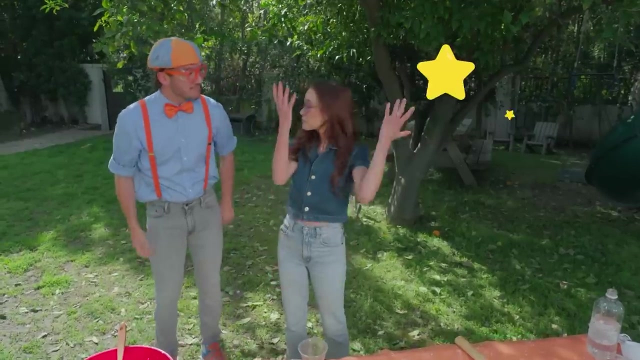 I know engineers build bridges and roads, but what does an aerospace engineer do? Well, aerospace means I study to help things fly through the air- Like an airplane, Woo-hoo, And like that paint can. And fly through space- Wow, that's amazing. Well, I definitely want to try this experiment. Let's go, Woo-hoo. 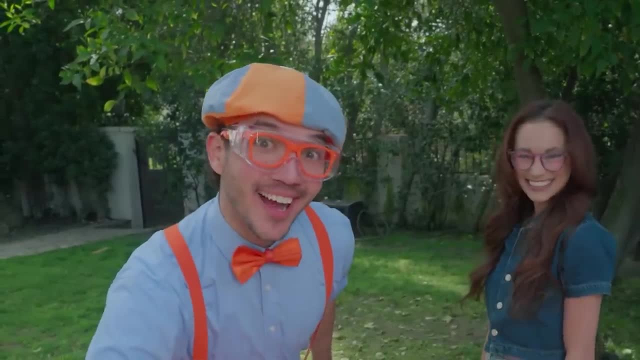 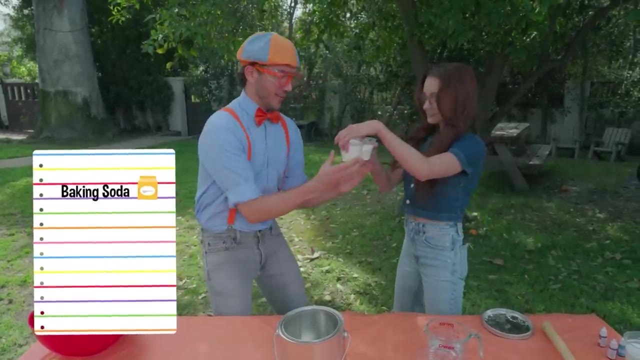 Blippi, are you ready? I'm ready, Are you ready too? Yeah, Awesome, Okay. Well, what do we need to do the experiment? We are going to need baking soda. Oh, okay, Some baking soda, and. 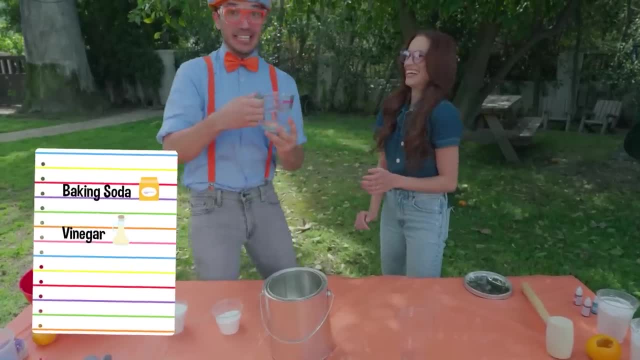 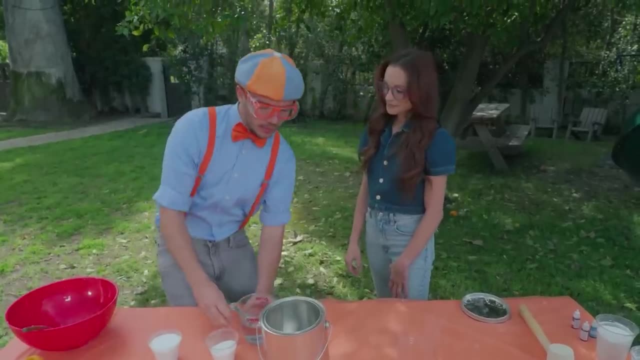 Some vinegar- Whoa, That's kind of smelly Whoa- And a paint can, And a paint can, That's right. Whoa, Wait a minute. Well, why will we need vinegar and baking soda to do this experiment? 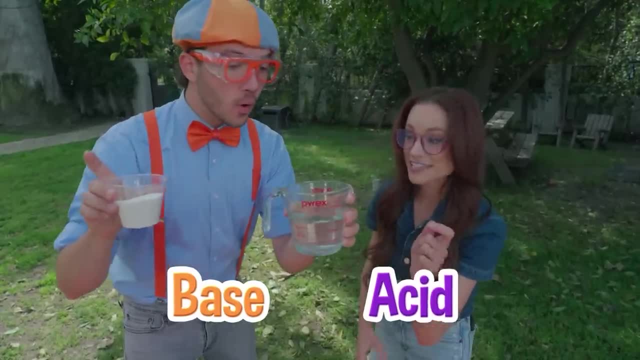 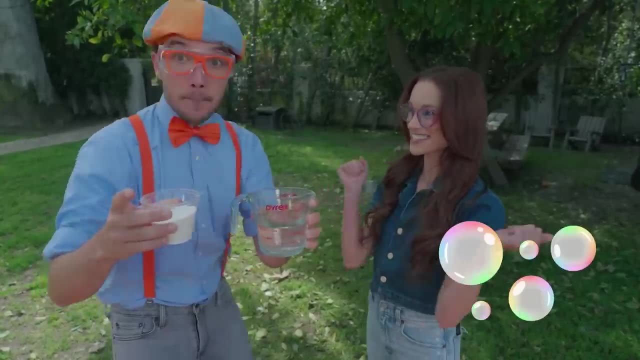 Well, baking soda is our base, Vinegar is our acid. When we mix the two together, you kickstart an acid-based chemical reaction that creates carbon dioxide bubbles, Bubbles, Yeah, Wait. and then the bubbles build up pressure, so it launches. the paint can like a rocket. 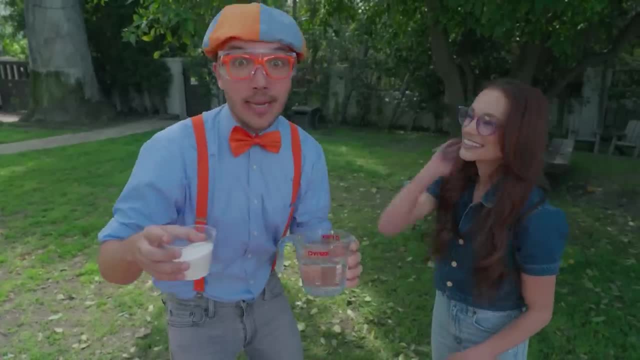 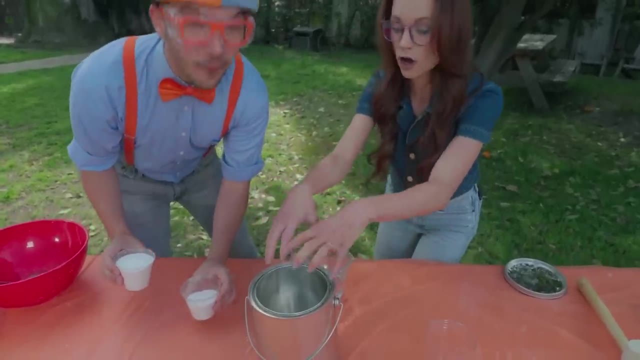 Woo, Exactly, Exactly, Okay. Well, I think we're ready to start the experiment. What's the first step? Okay, So first you're going to want to put your baking soda in the paint can Just pour it all in. 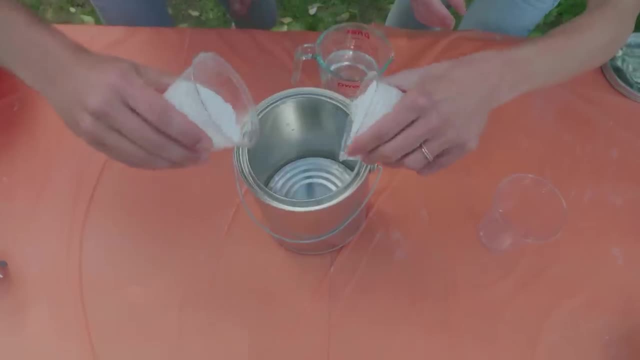 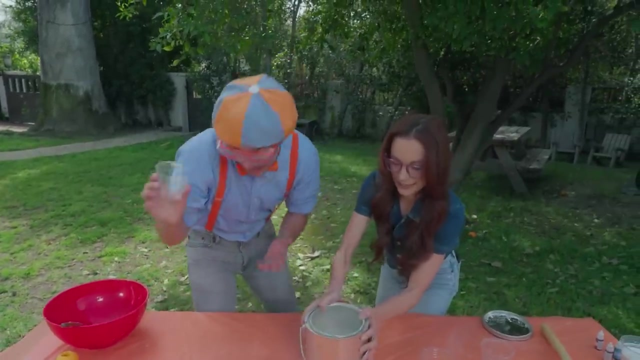 Okay, Here, Can you help me? Yes, absolutely, Here we go. Woo-hoo, It's snowing. Snowing in the paint can? Whoa? Oh, It's a little messy doing science. Okay, Now you want to put your vinegar in this cup. very carefully. 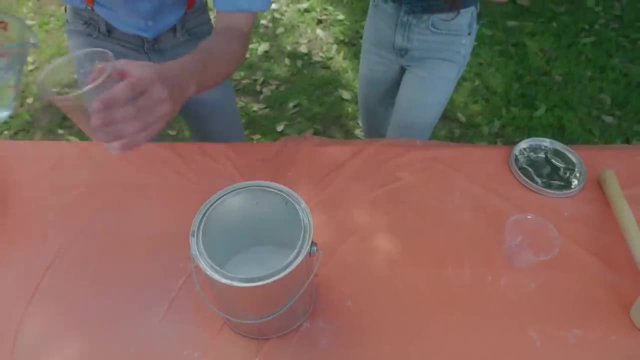 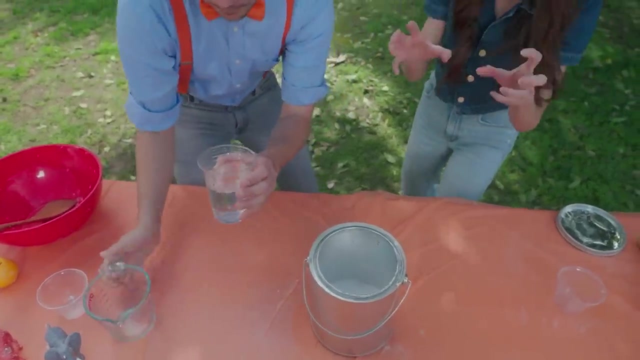 Oh, and then we put the cup inside. Exactly. Okay, Here we go. Don't want to spill any on the baking soda before it goes in. Yes, Be very careful. We don't want to kickstart the acid-based chemical reaction too soon. 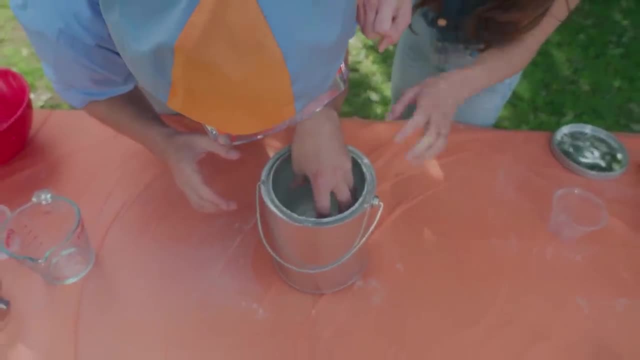 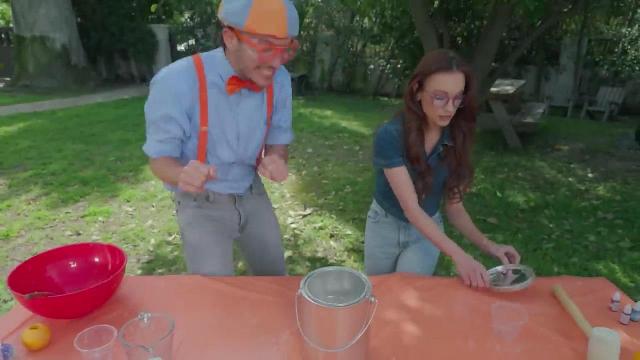 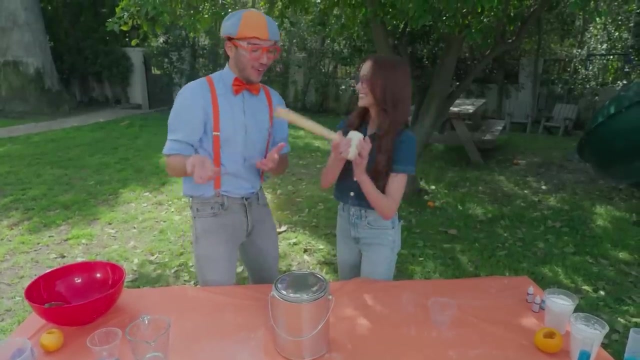 So just softly nestle it into the baking soda, Just like that, Exactly, Whoa, Yes, Looks pretty steady, Perfect. Now for the final step, The fun part. Okay, We're going to hammer on the lid. Oh, that's why you were hammering before. 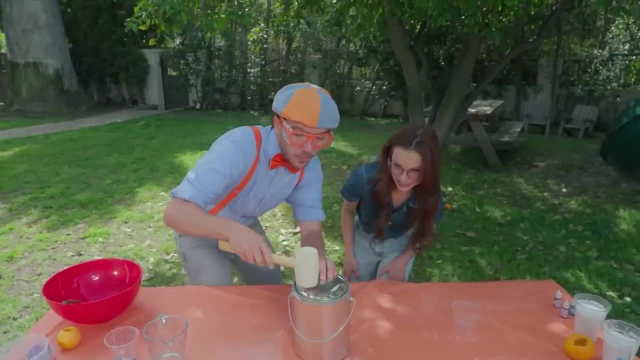 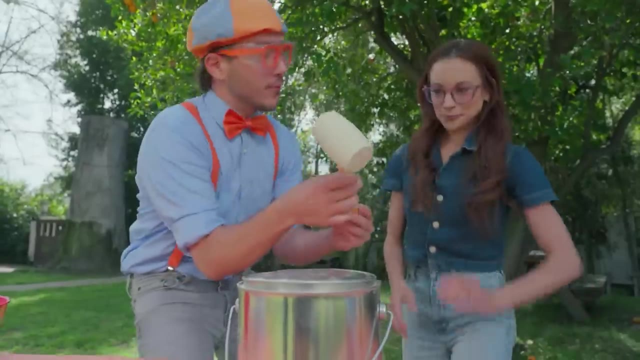 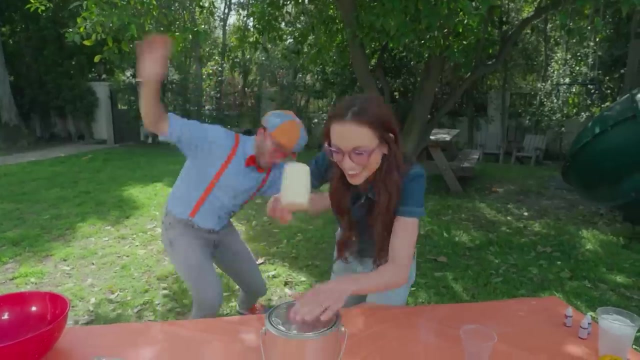 Exactly Okay. Here we go. Is this okay? Yep, Perfect, Emily, you want to hammer some? Absolutely, You need to put a little bit of oomph behind it. Oomph Whoa, That's some oomph Whoa. 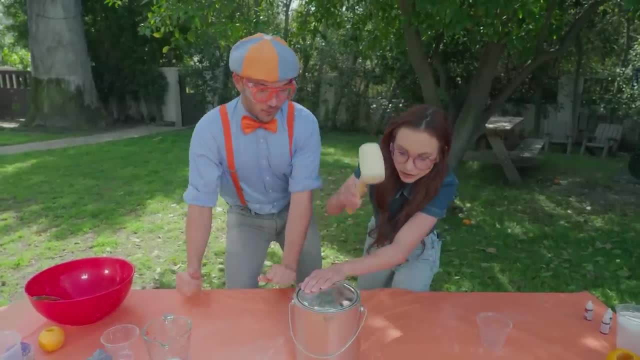 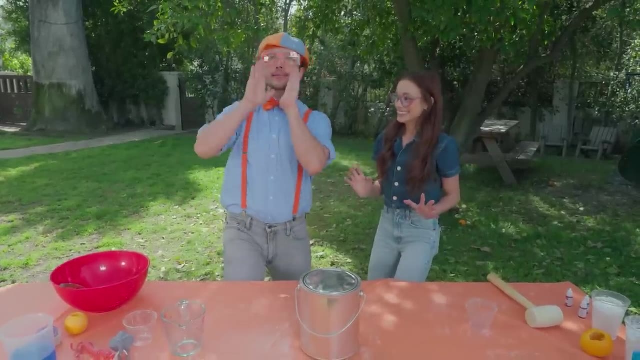 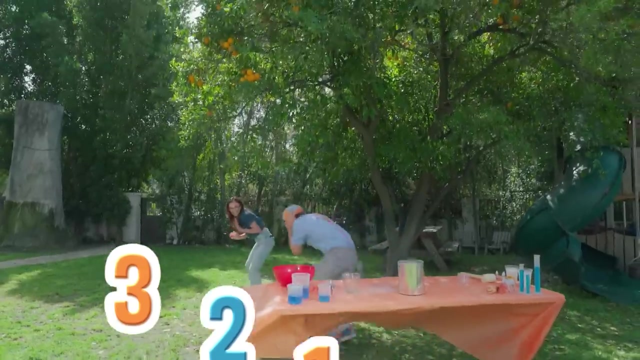 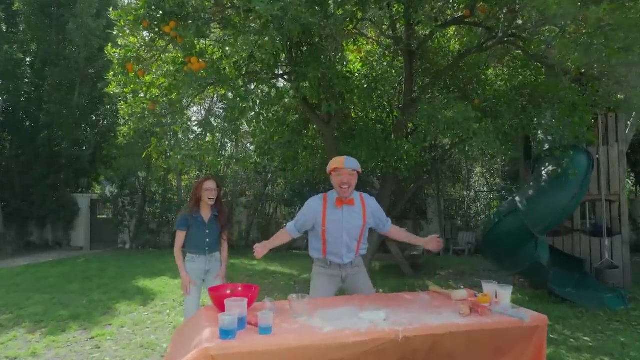 Okay, I think it's ready. Yeah, Okay, And now we just flip it over Exactly. Okay, Everyone, take ten steps back. Here we go, Three, two, one, Did you see that? Yeah, Flippy, do you want to see what was going on inside the paint? can? 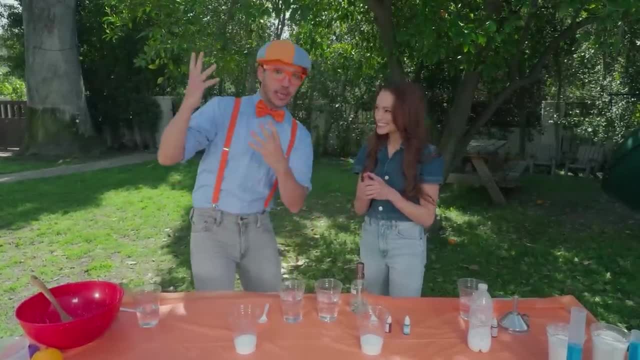 Whoa, That would be awesome. Yeah, we saw it launch like a rocket, but I want to see those carbon dioxide bubbles: Boop, boop, boop, boop, boop, Okay, Okay. so what do we need to do? 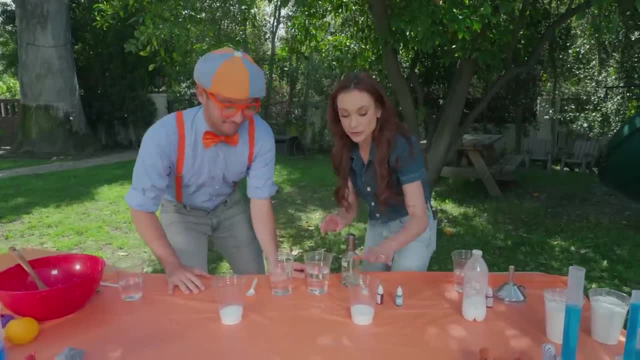 We can make them right here. So we have vinegar, that's our acid, and we have baking soda- that's our base. So what we're going to do is add our food coloring first, because everything is more fun in color. Whoa. 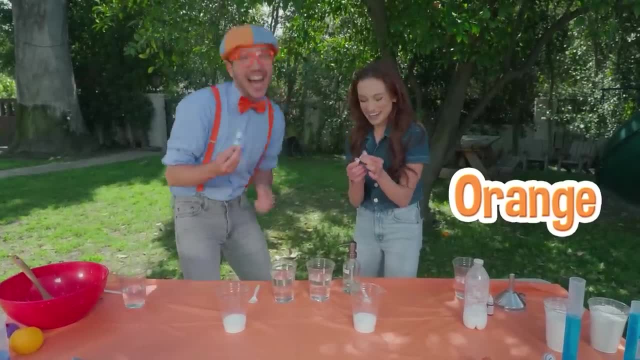 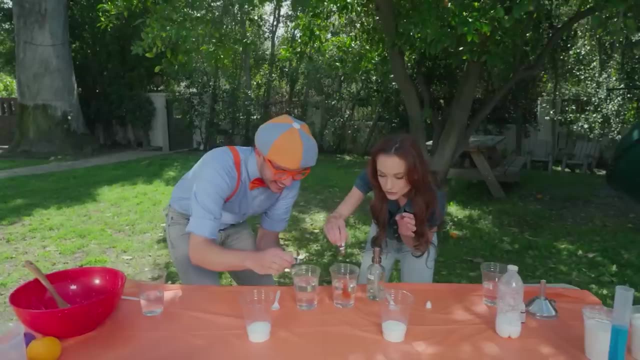 We'll give you blue And you have orange. I have orange. Yeah, Huh, I wonder why we're using those two colors. I thought they might be your favorite. Yeah, So go ahead and add a shot. I'm going to add a few drops, just like that. 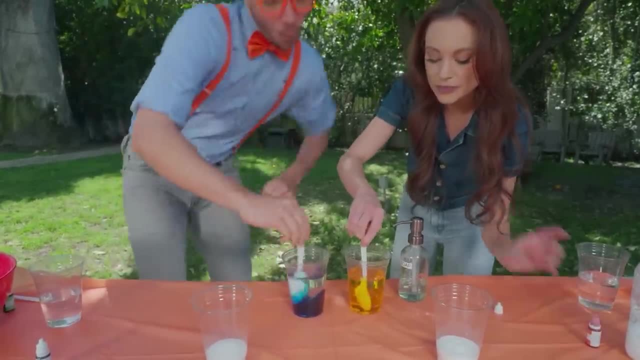 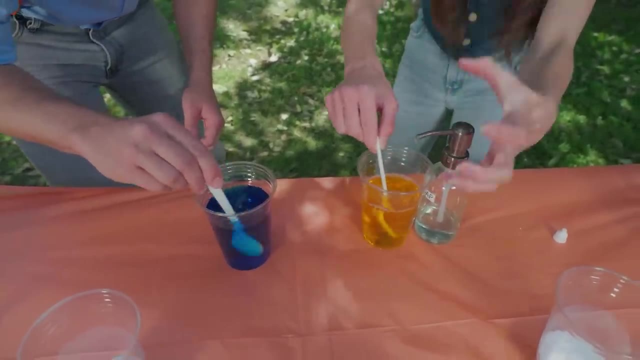 and let's stir it in. Okay, Give it a good stir. Now, in one of these I'm going to add some soap. My hypothesis is that the soap is going to trap those carbon dioxide bubbles and make this one a bit more frothy and soapy. 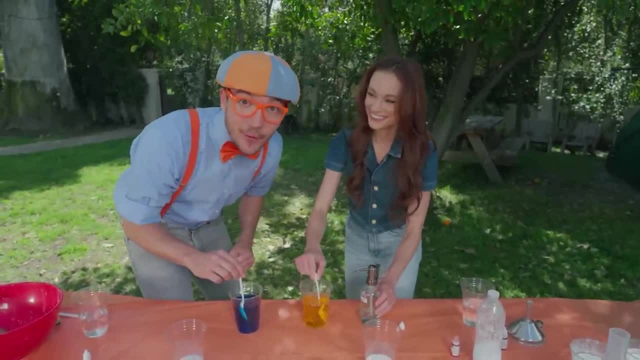 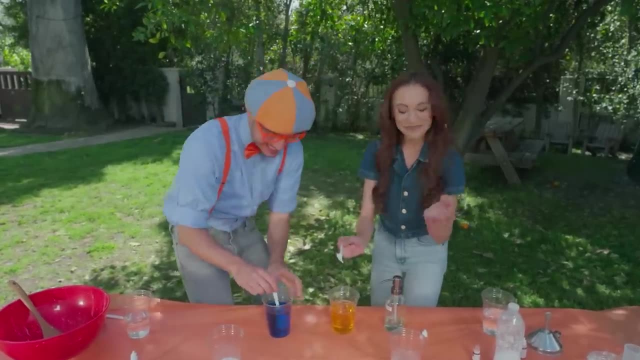 Whoa Hey, have you heard the word hypothesis before? Yeah, it's a really long word for basically a guess, And, Emily, I think you made a really good guess, I think, so Let's test it out, though, Okay. 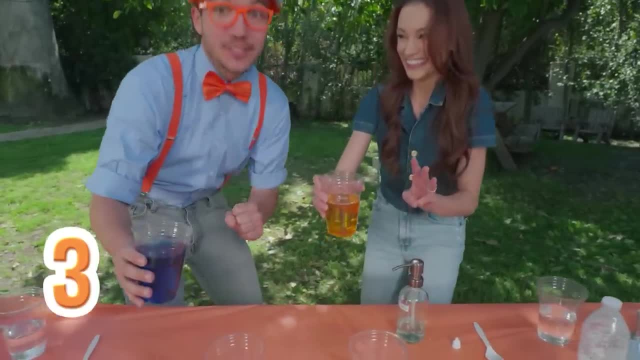 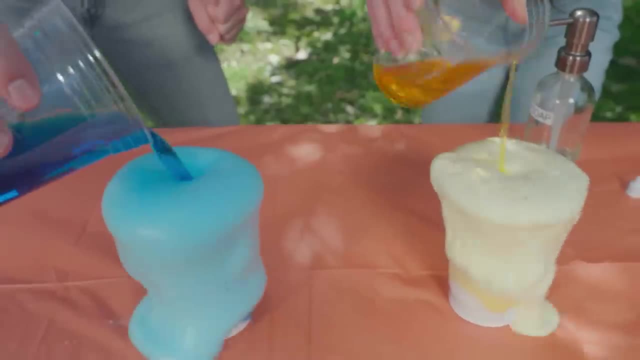 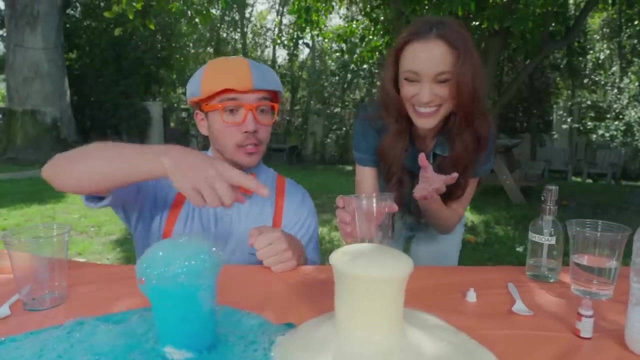 Okay, here we go, Ready: Three, Two, One, Whoa, Whoa. Check it out. Do you see how mine looks a little bit more frothy? That's the soap trapping those carbon dioxide bubbles. Yeah, it looks like yours has a lot of teeny bubbles. 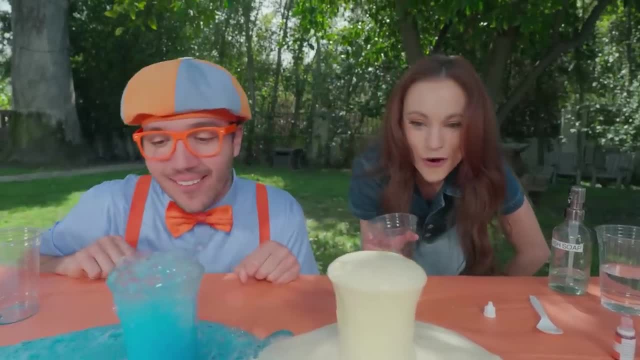 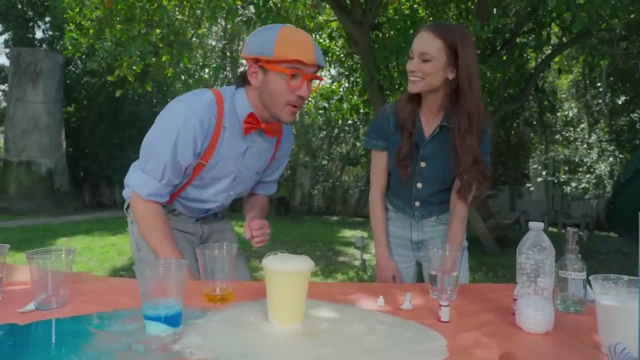 and I have really big bubbles. Exactly Whoa. that's cool. And, Emily, we used this experiment using cups. could we use a different container? Absolutely we could. Oh, what about that water bottle? This would be perfect. 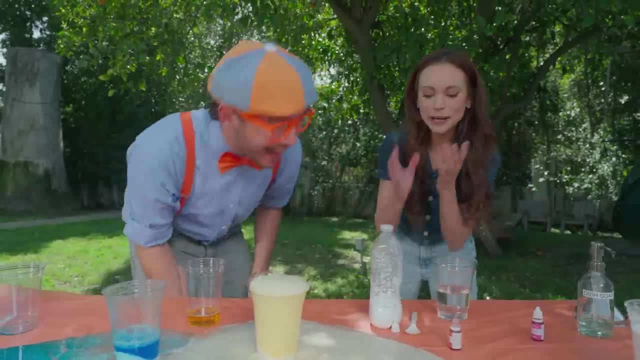 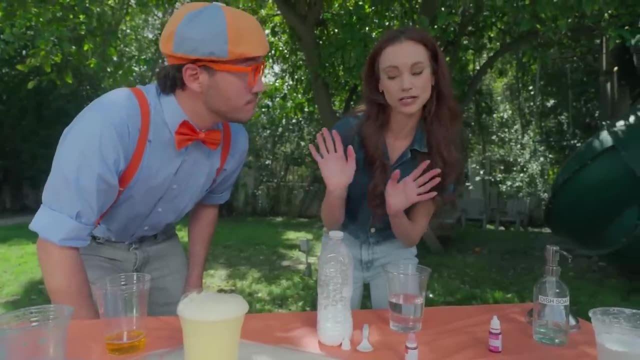 Huh, I wonder how the bubbles will shoot out of that. I know my hypothesis is because this one is going from a large area to a small area, it's going to shoot up faster and maybe go a little higher. Hmm, another good guess. 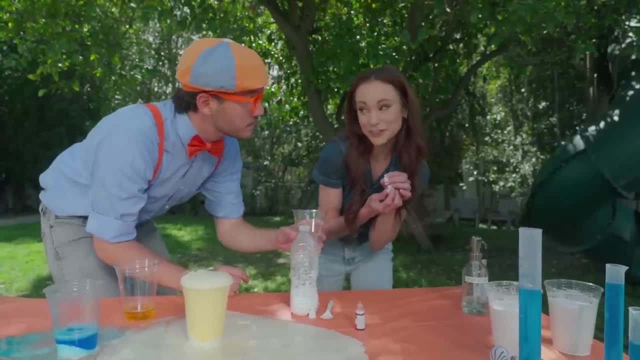 We've got to test it. Oh, and what color should we make this? Well, my favorite color is pink. Ooh, Can we make it pink? Yeah, let's make it pink. One, two, three. There we go. 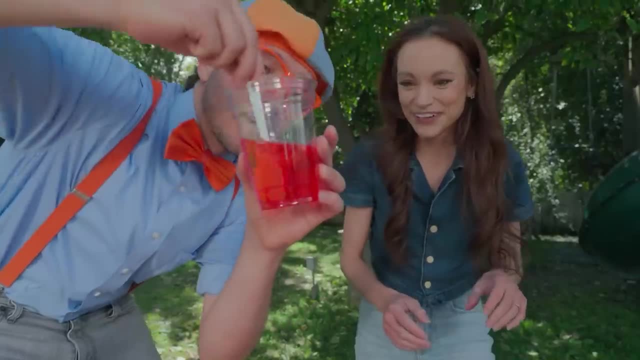 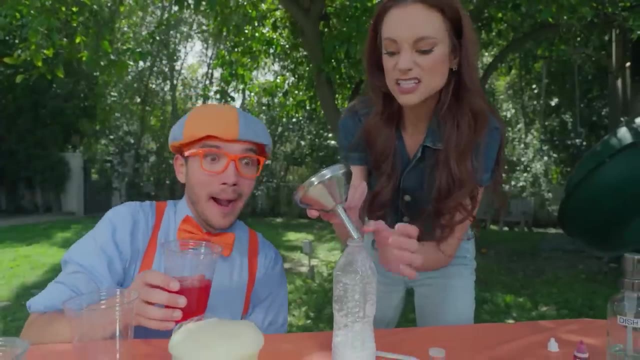 Stir that in Whoa, it's like a pinky red color. Oh yeah, Oh, that's going to be some fun bubbles, Okay, so now we're going to pour it in and let's see what happens. Let's test that hypothesis. 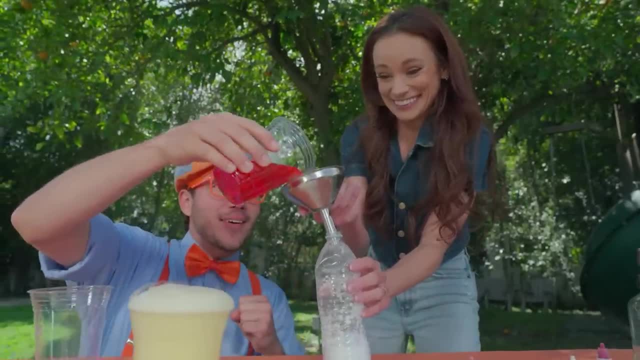 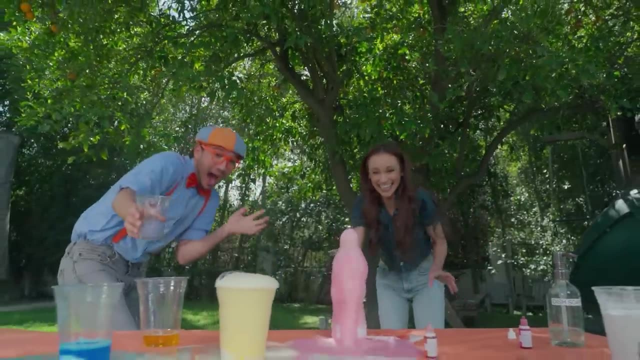 Okay, get ready, These are going to be some big bubbles. Woo-hoo, Whoa, Whoa. Your hypothesis was right. It shot up higher, didn't it? Yeah, That was great. Whoa, that was really cool. 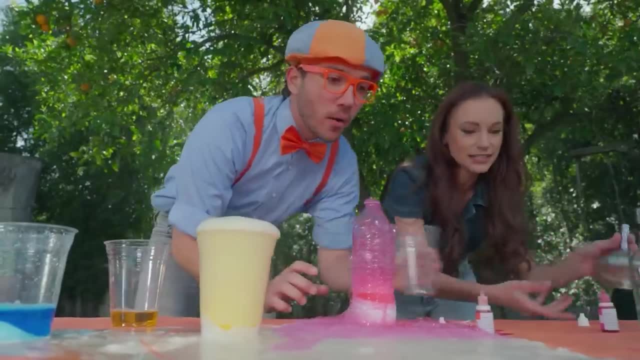 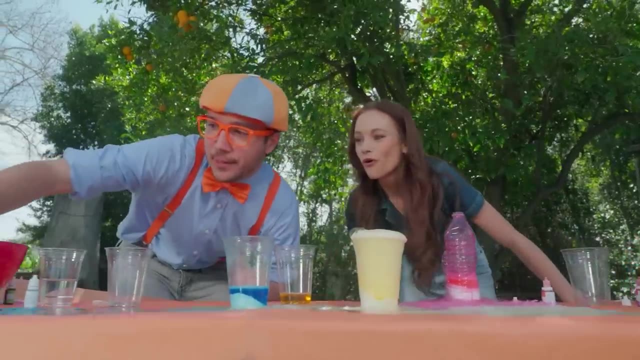 Bubble launch And now it looks so pink. look at that. Whoa, Yeah, we have some pink and we have some orange and some blue. Woo, Look, Emily, We have a fun little elephant in some blue water, just taking a bubble bath. 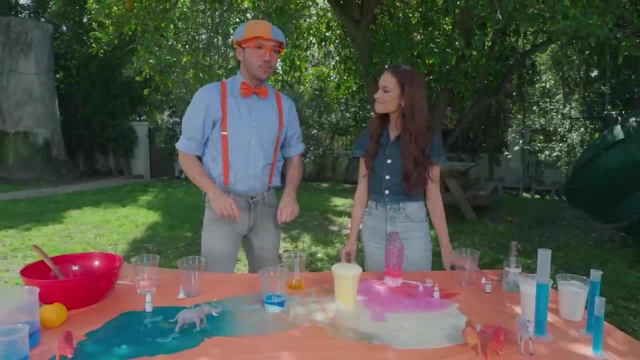 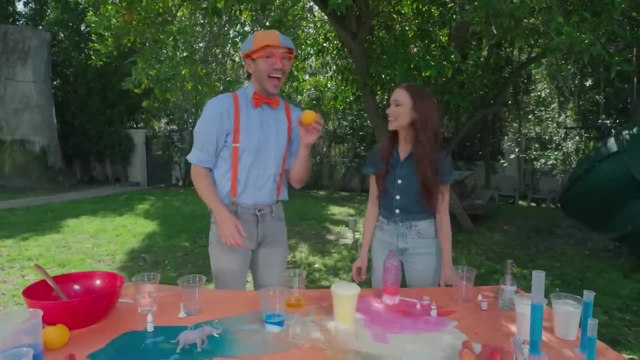 Oh, wait a minute. We tried a cup and a water bottle. What if we try something a little bit silly? Okay, What did you have in mind? An orange, Let's try it. Yeah, I love the color orange and I love eating. 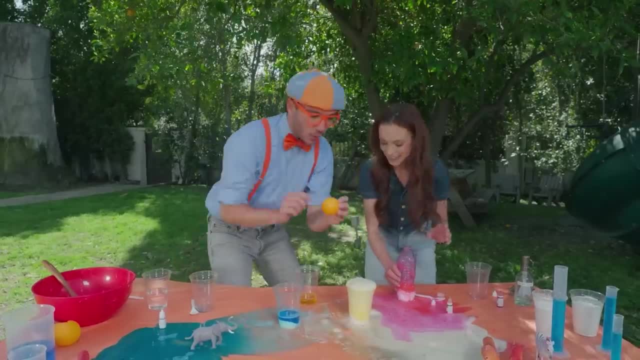 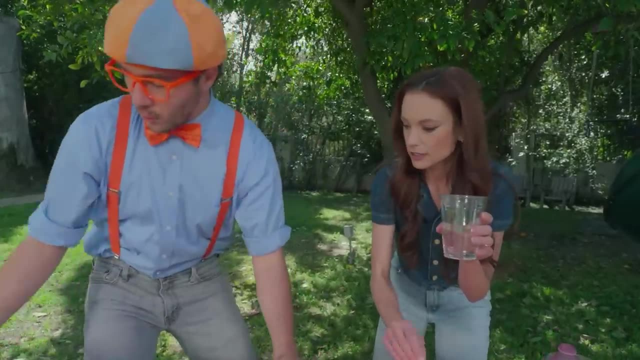 The fruit in orange. Okay, so we have an orange and there's some baking soda inside And here's some vinegar for you. Okay, thank you. And this one I want to be extra silly, so let's make the vinegar green. 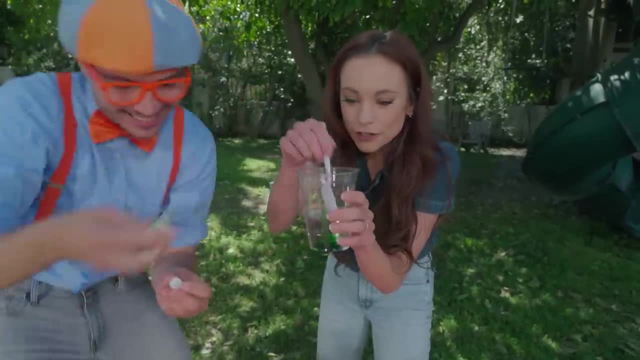 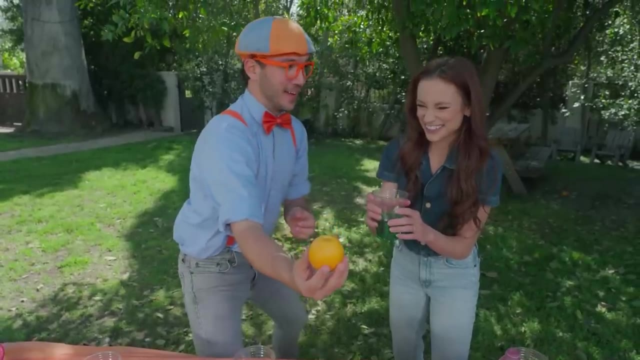 Oh, I like it. We haven't done green yet. Whoa, Perfect, I'm going to stir that up. All right, let's see what this one looks like. Okay, I don't know what it's going to look like. 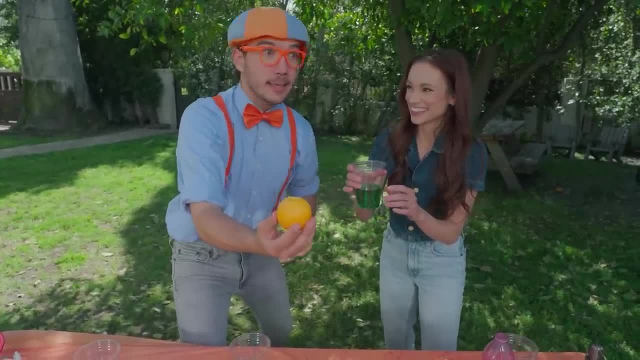 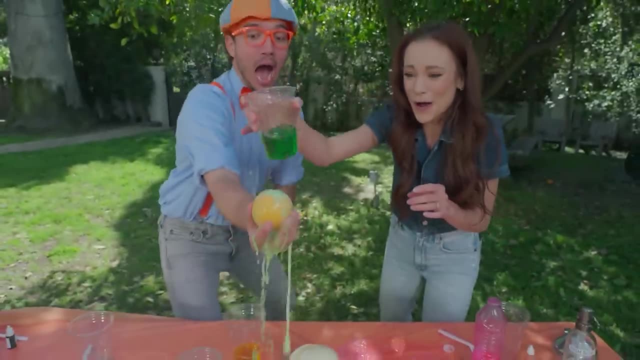 I'm going to try to hold it. My hypothesis is that this is the one. It's going to be messy. Three, two, one Go, Whoa, Whoa, Whoa, Whoa. It's so fizzy. 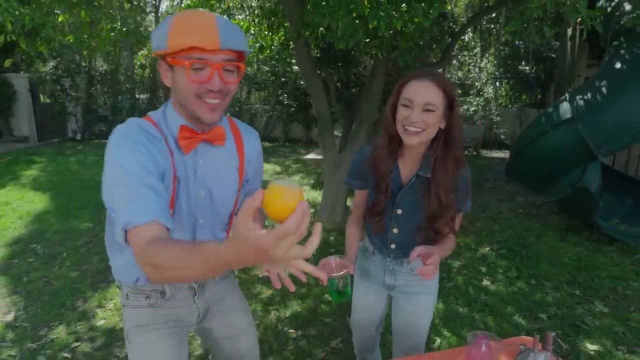 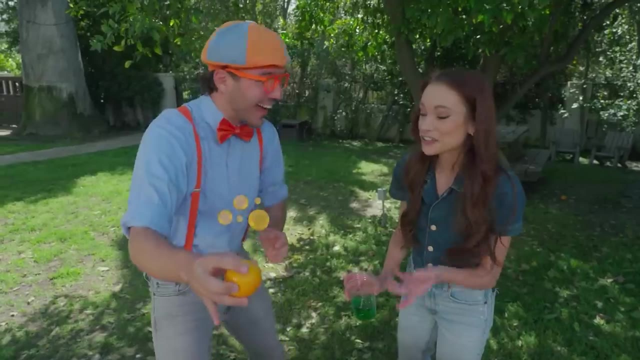 Whoa, Emily, that was awesome, That was great. Whoa, yeah, Look at that. So many bubbles, Those carbon dioxide bubbles, went everywhere. That's a great acid-based chemical reaction right there. Well, this was some fun experimenting. 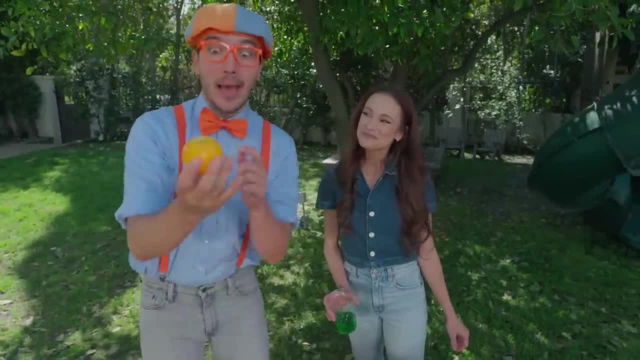 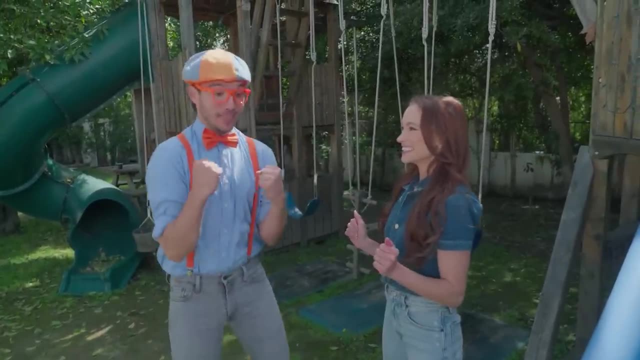 Do you think we could do another one? I think so. Okay, I'm going to go clean up my hand. Flippy, are you ready for the next experiment? Mm-hmm, I'm really excited, but I think we should take a little break first. 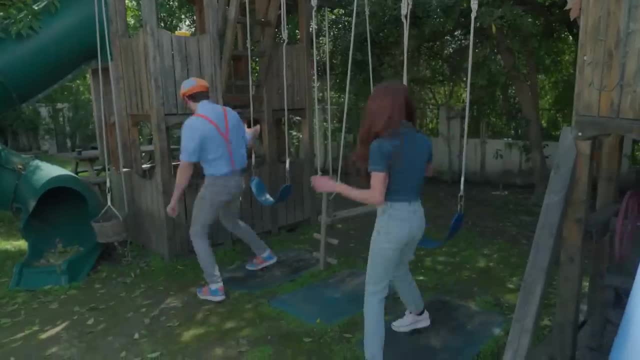 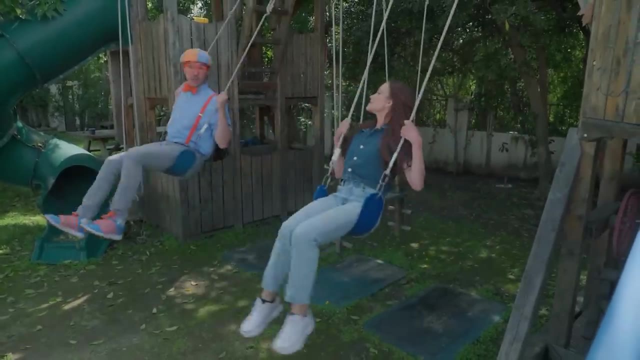 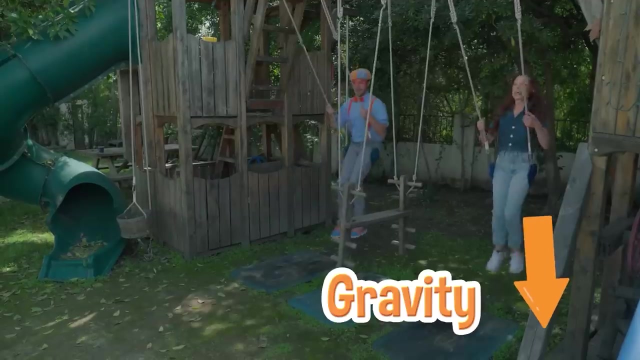 And look a swing set. Come on, Let's go. Whoa, I just love swinging, But, Emily, Yeah, Is there something scientific about swinging? Oh my gosh, yes, There's science. all around us With swings, gravity is bringing us back down. 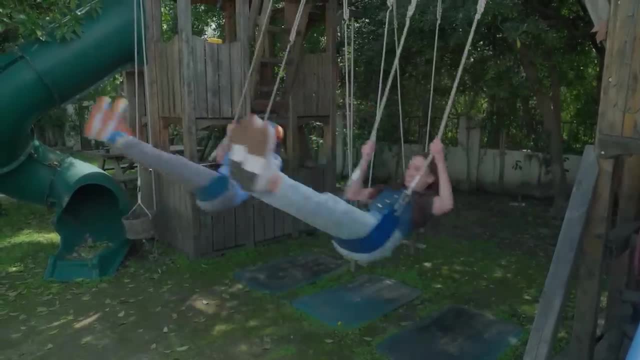 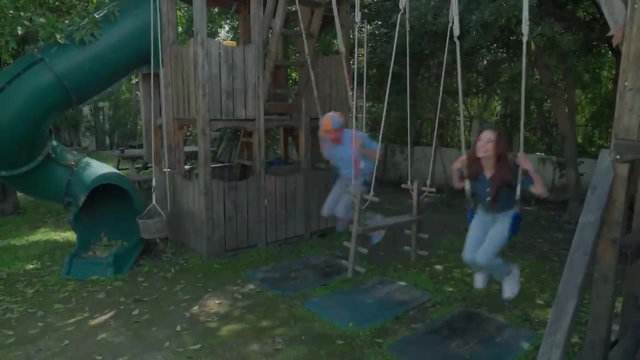 and our legs are giving us momentum to bring us back up. Yeah, and my legs are really strong from dancing, so I can go really high on the swing. Whoa, good thing we have gravity to bring me back down, or else I might fly all the way to the moon. 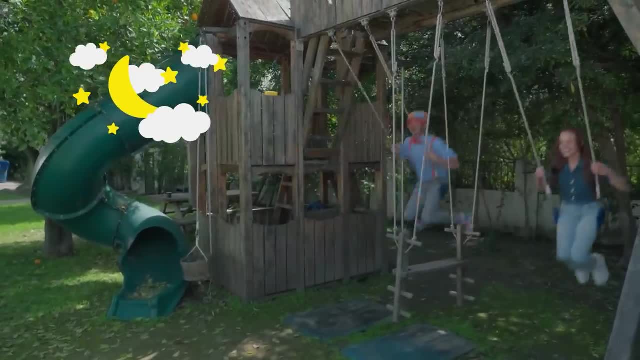 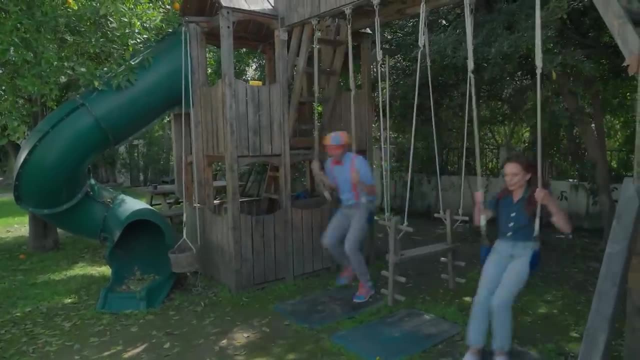 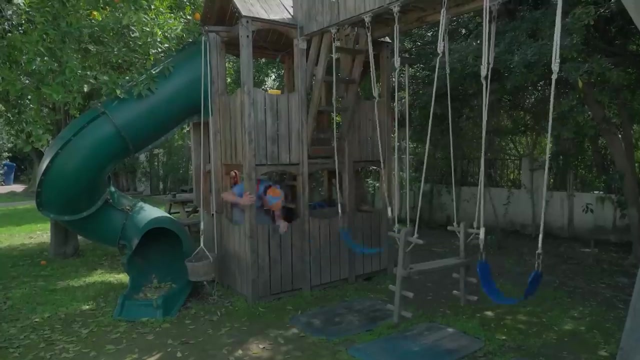 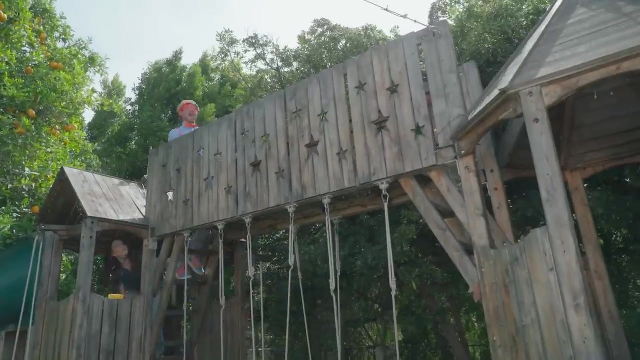 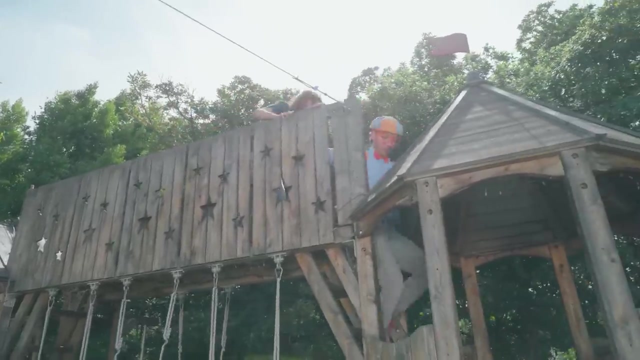 That would be fun. Oh yeah, Astronaut Flippy, here I come, Woo-hoo. Oh, Emily, I have an idea. Follow me. Okay, Here we go. Wow, I had so much fun taking a break. 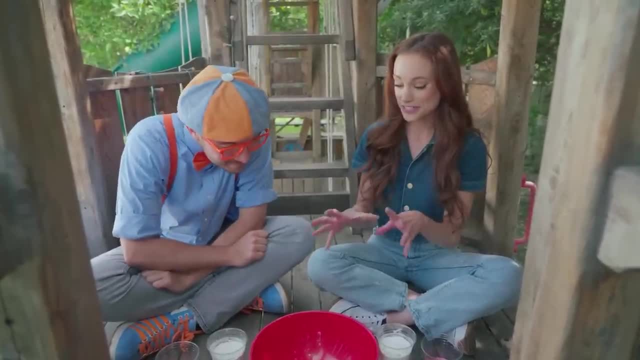 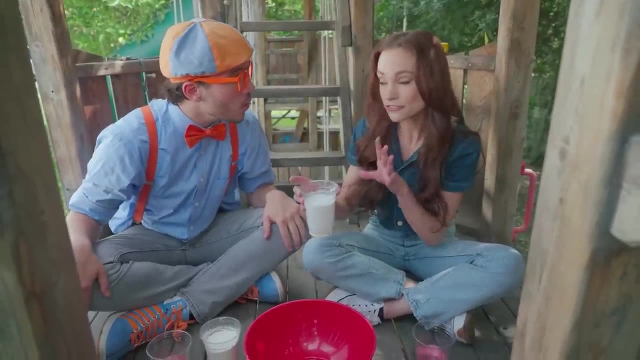 But, Emily, I'm ready for another experiment. All right, We are going to make oobleck, Oobleck Fun. Oobleck is a non-Newtonian fluid and all you need for this. you can make this at home. 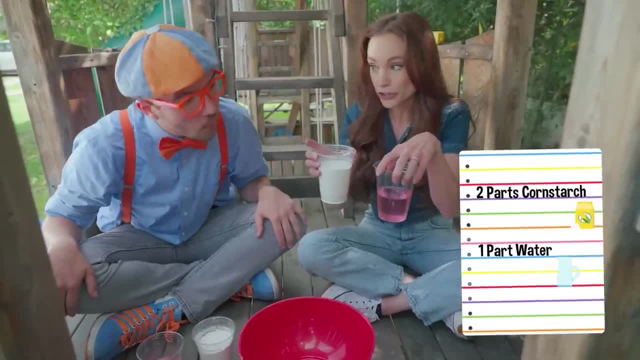 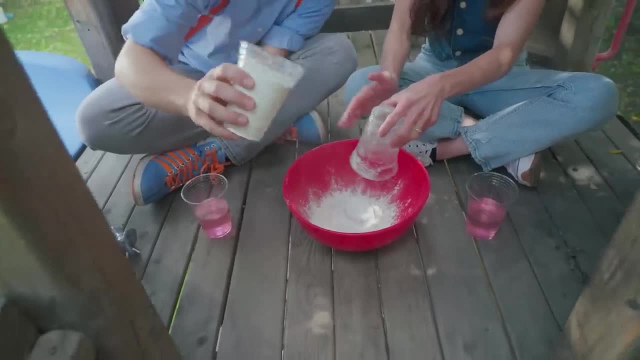 is two parts cornstarch to one part water. Ooh, So let's go ahead and mix those in. Wow, Put your cornstarch in here. Okay, Go ahead. Cornstarch, Just like so Good, good, good. 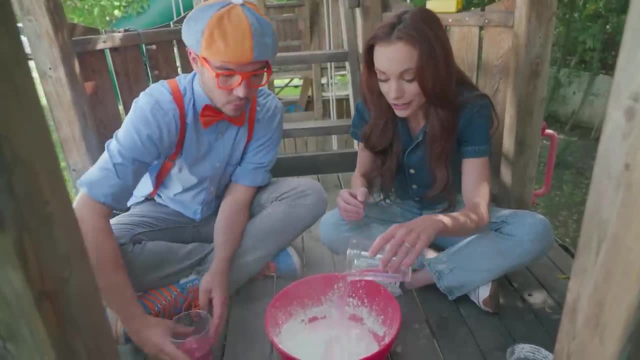 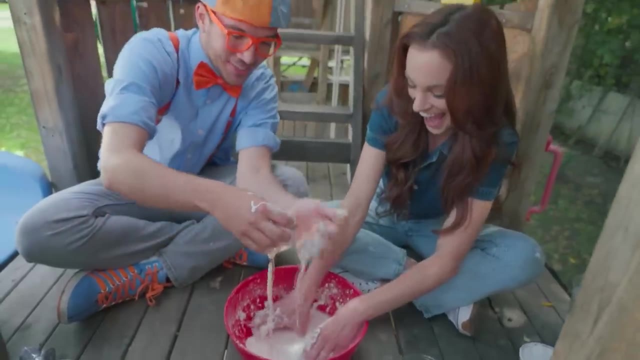 Oh, it's snowing. Whoa, Now add your water. Okay, Just like that. And you're going to want to just get your hands in here? Whoa, This is really fun mixing it up with your hands. And you said it was a non-Newtonian fluid. 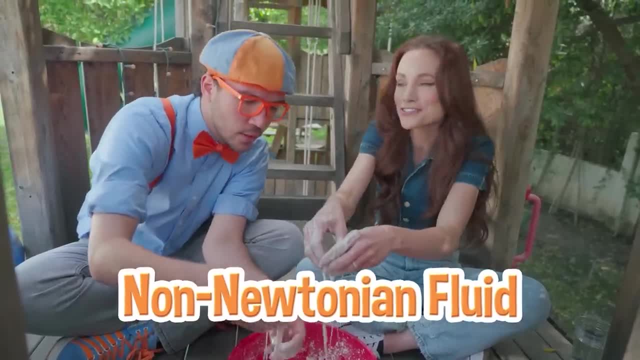 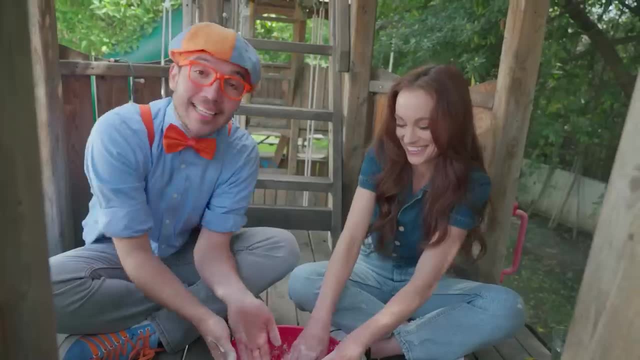 Yes, Whoa, So a non-Newtonian fluid is just a special name for a fluid that doesn't follow the normal fluid rules. Oh yeah, So a normal solid has its own shape and a normal liquid or a fluid takes the shape of whatever container it's in. 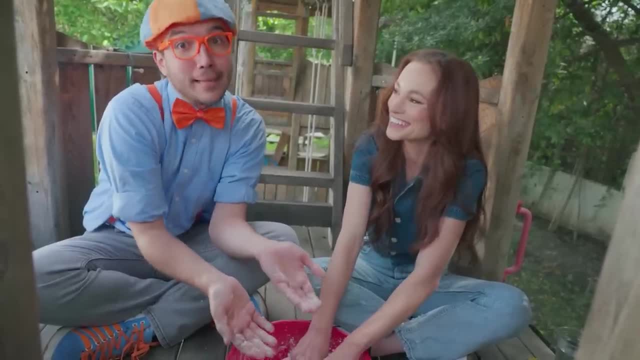 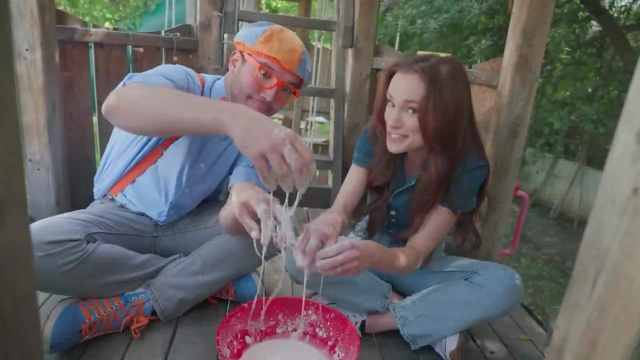 So if you have water in a cup, the water is shaped like the cup, Exactly, But oobleck, because it's a non-Newtonian fluid, sometimes acts like a liquid, but it sometimes acts like a solid, depending on what we do to it. 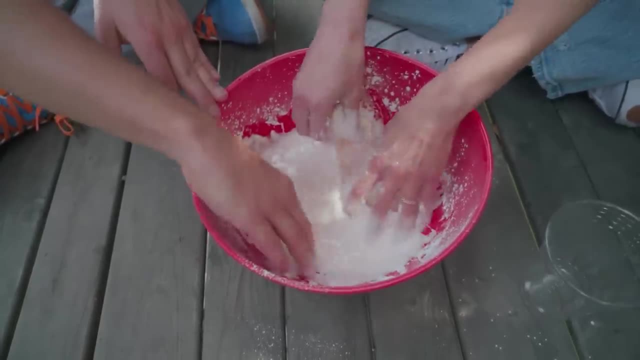 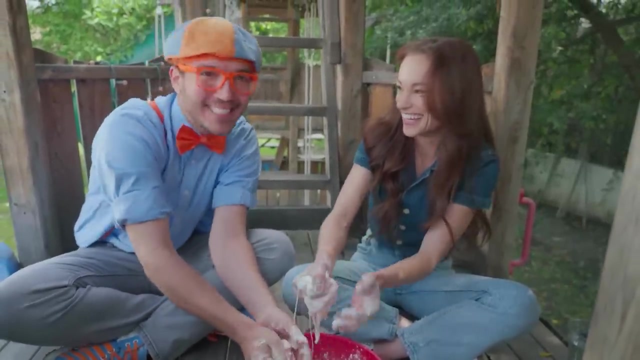 Oh Whoa. So are there other kinds of non-Newtonian liquids? Exactly, So one you might be familiar with is ketchup, Ketchup, Yum, I love that on my French fries, And when you're trying to get ketchup out of the bottle, 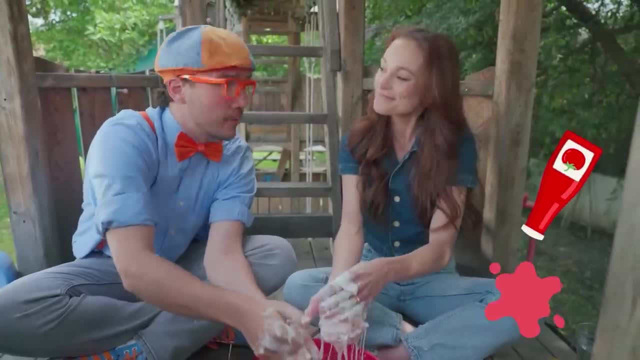 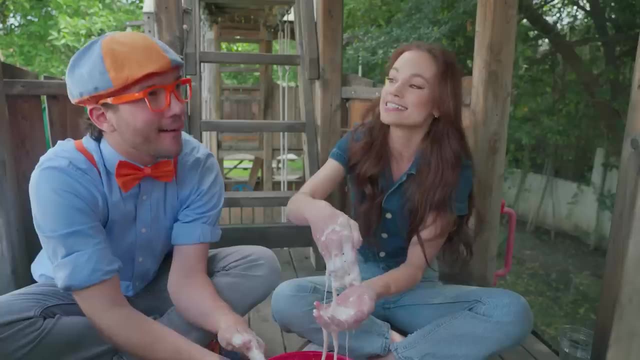 what do you usually do? You normally need to tap the end of it a little bit, Exactly Because, ketchup, when you hit it, when you add force to it, it acts more like a liquid. Oh, And when you don't hit it, when you're not doing anything to it, 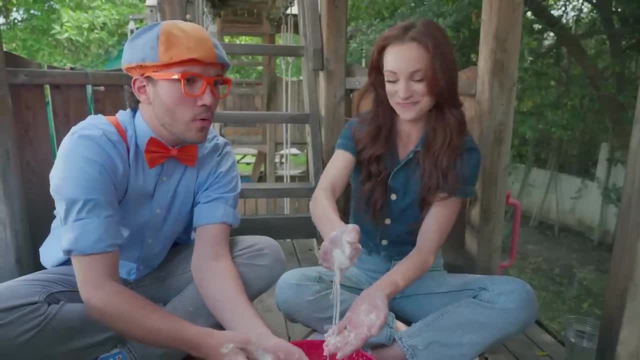 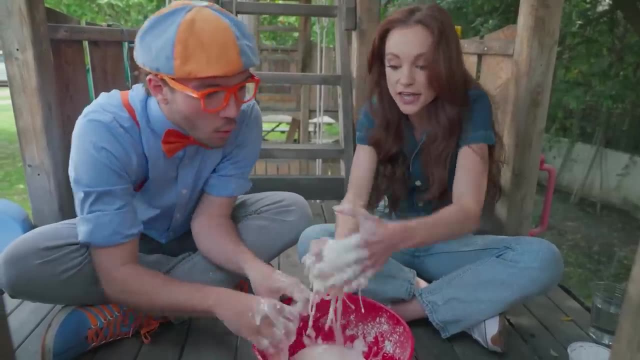 it acts more like a solid and it's harder to get out of that glass bottle. Whoa, that's so interesting how it can be a solid sometimes, or a liquid sometimes, Exactly Just like oobleck. So watch this When you squeeze it together. 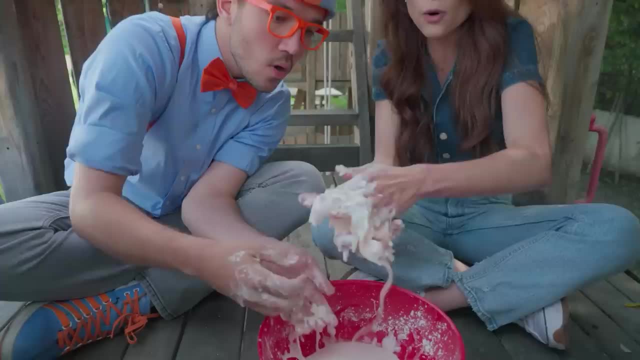 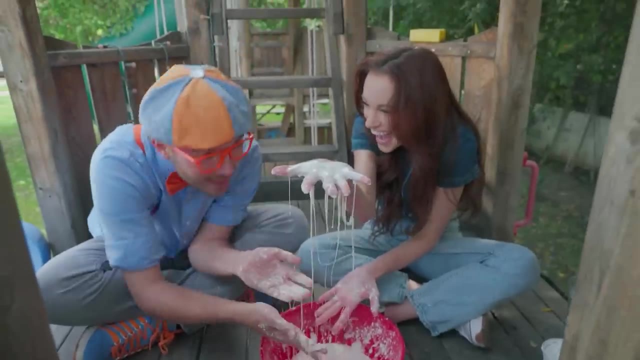 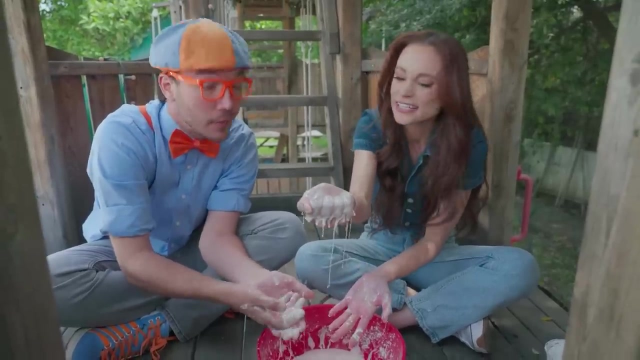 squeeze, squeeze, squeeze. it acts like a ball, But watch this: As soon as I stop squeezing it, it acts like a liquid flowing through my fingers. Whoa, it melts. That's so cool. Whoa, And why is it called a non-Newtonian fluid? 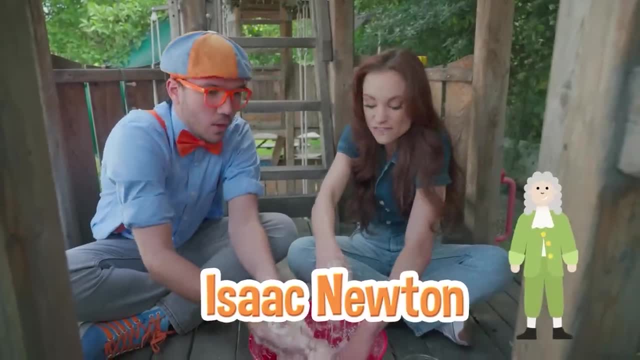 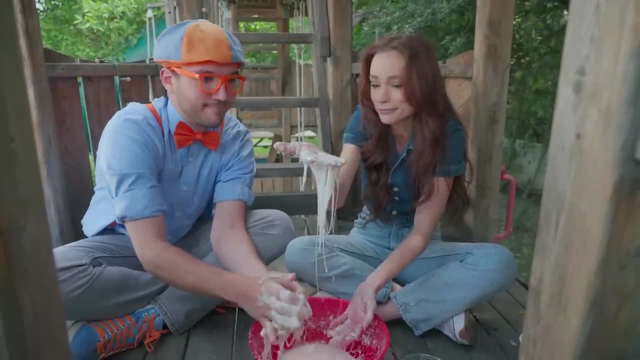 Yeah, That's a long name. That is a long name. So Isaac Newton was a physicist and a mathematician and he set up some rules for fluids And this doesn't really follow them. It likes to break the rules. Yeah, and I've heard of Isaac Newton. 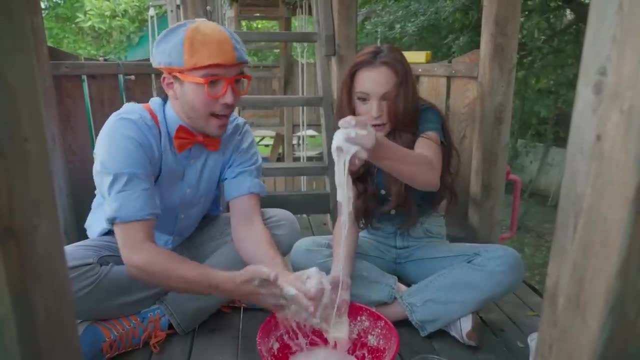 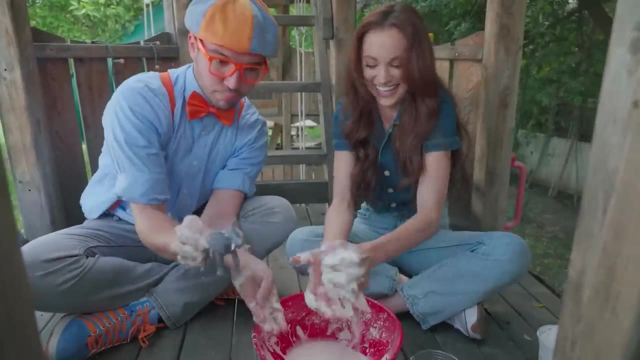 That's so cool that he named this fluid. Yeah, Whoa. Oh, I have an idea. How about you make a little ball again, and I think our friend Mr Elephant wants to play in the oobleck. Here we go. 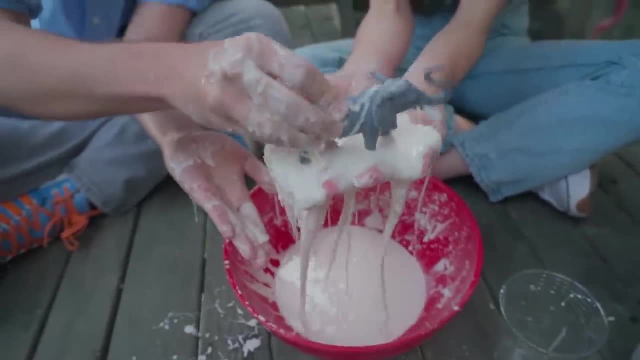 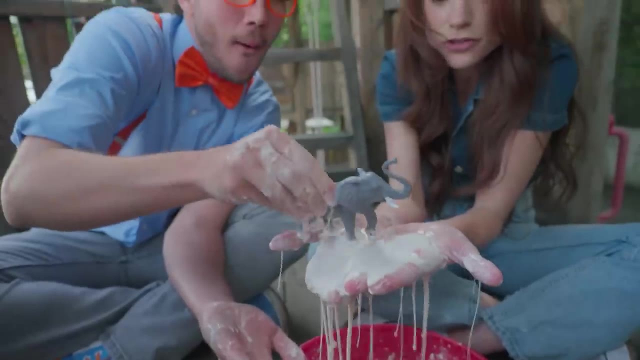 Whoa, Uh-oh, He's getting stuck. Well, that's okay. Yeah, If he just moves around a lot, he doesn't get stuck. See, He's just walking in over the oobleck. If he stomps on the oobleck, 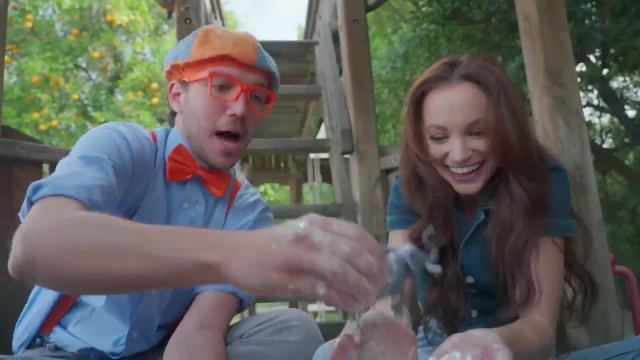 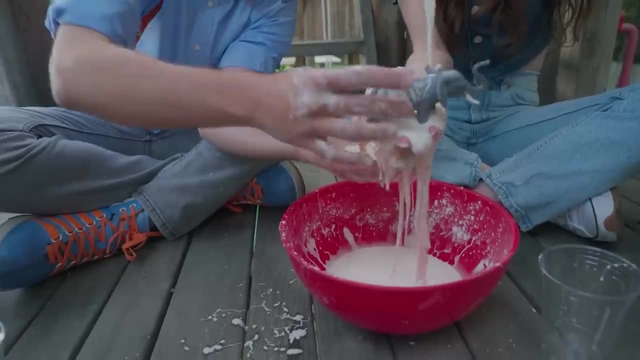 he can stay on top. Look, Stomp, stomp, stomp, Stomp, stomp, stomp. Yeah, But if he's not stomping, he'll sink like water. Here we go, Whoa, Whoa. 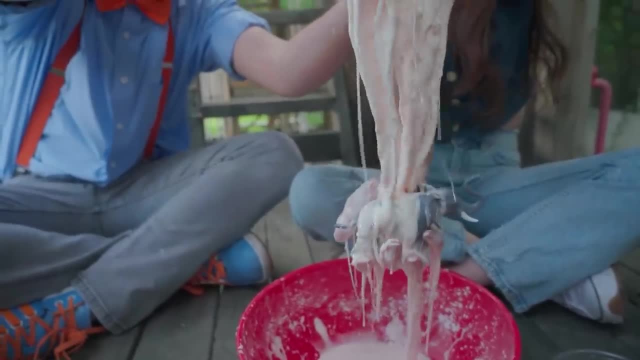 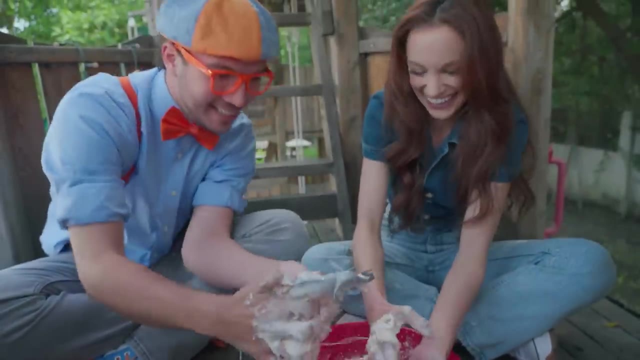 Whoa, Whoa, Whoa, Whoa, Oh, Oh, Oh, Oh, Like well, it looks like Mr Elephant needs to go take another bubble bath. Oh, Emily, this oobleck is super fun, Woo-hoo. 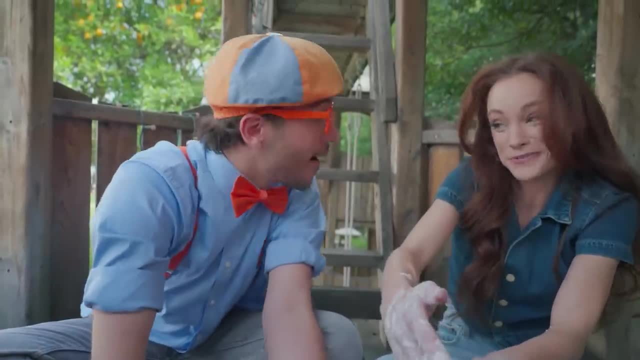 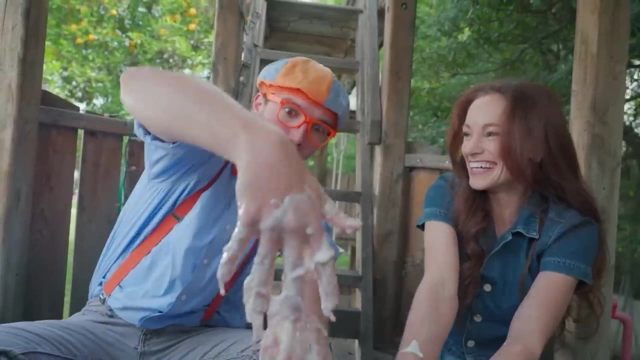 Okay, Blippi, now that you know how oobleck works, I have a surprise for you. You have a surprise for me? Yep, Well, where is it? Go ahead and slide down that side. Okay, Here we go. 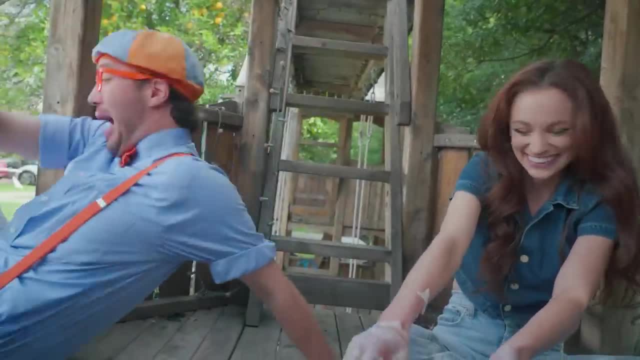 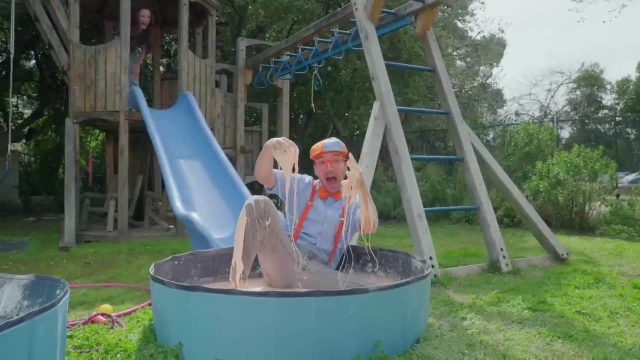 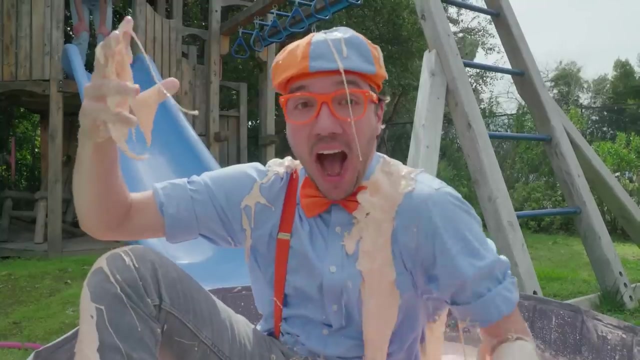 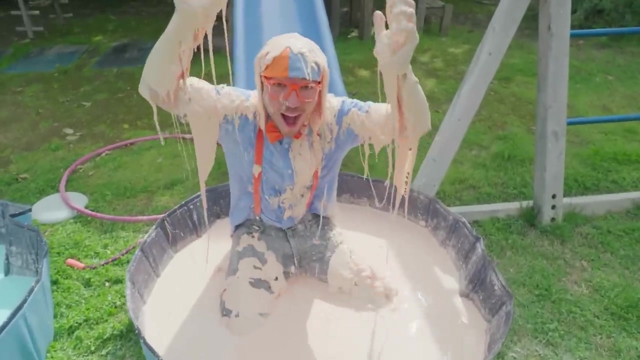 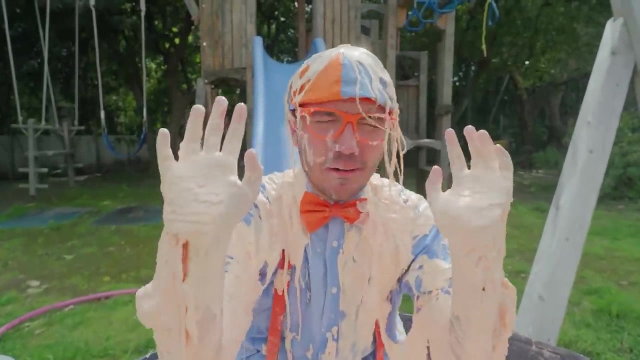 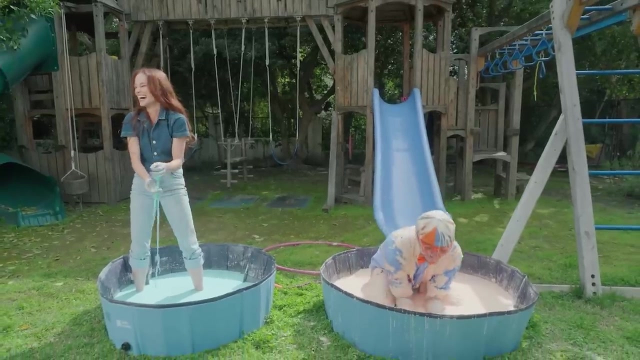 See you at the bottom. Woo-hoo, Ha-ha. This is an oobleck, This is oo-blippi, Blippi, Blippi. that's a corny joke, A cornstarchy joke. Whoa, I had so much fun today.